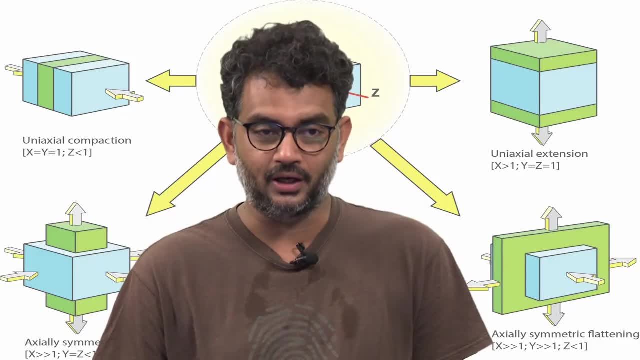 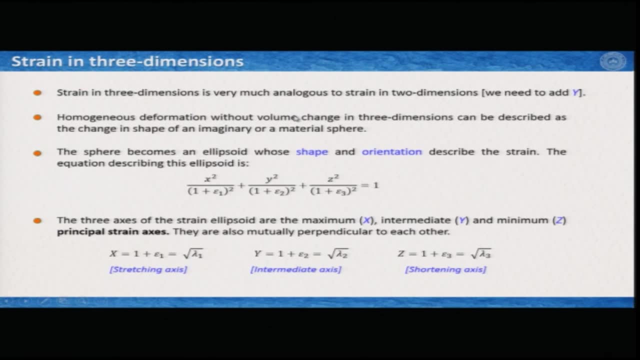 deformation, from where we will switch to vorticity and conclude the lecture. So strain in three dimensions is very similar to what we have learnt when we understood the strain in two dimensions. There we had x and z, and this time, because we will be dealing 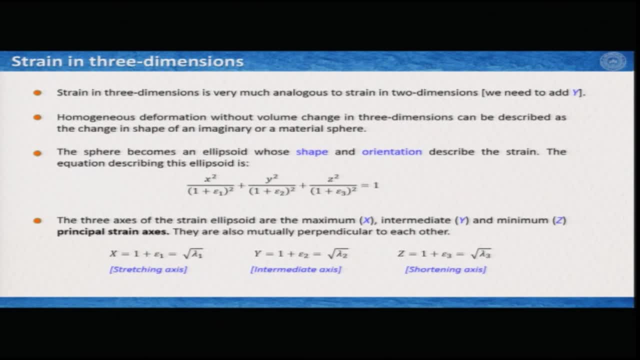 with three dimensions. we will add y, So homogeneous deformation without volume change in three dimensions. generally, like we described previously with strain ellipse, this time we will use the strain ellipsoid, which is a shape change from an imaginary or a material sphere. Now the sphere becomes an ellipse, so we have to describe its shape and orientation. 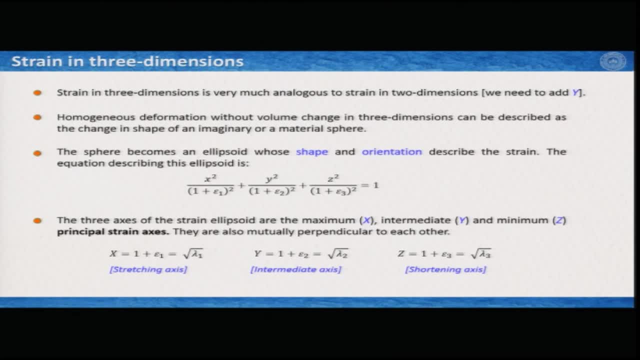 to describe the strain, and the ellipsoid can be described by this equation. So the three principal axes of strain are here, and then it is a Cartesian coordinate system: x, y, z. So the three principal axes of strain are the maximum, intermediate and minimum principal. 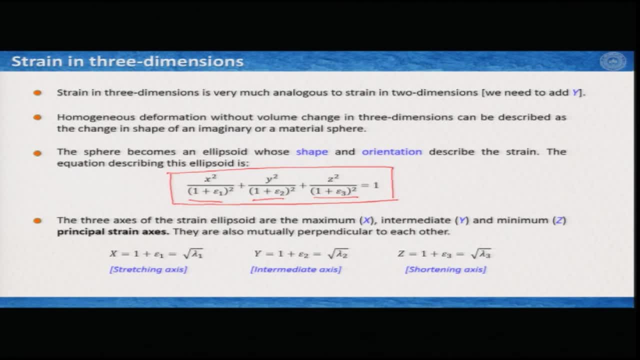 strain axis. So they are also mutually perpendicular to each other. and like we have described the x and z axis in the 2D, we have to add here the intermediate axis, which is y equal to 1, plus epsilon 2 or root over of lambda 2.. The other two remains the same, that is x equal. 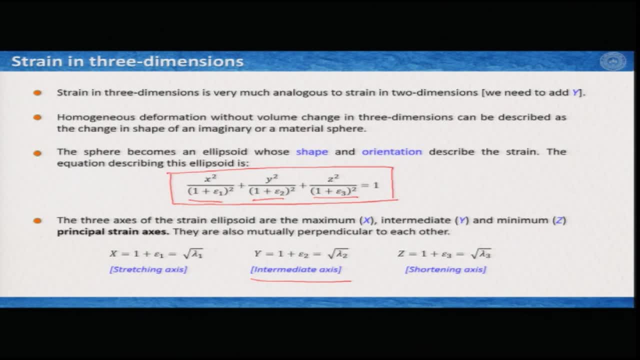 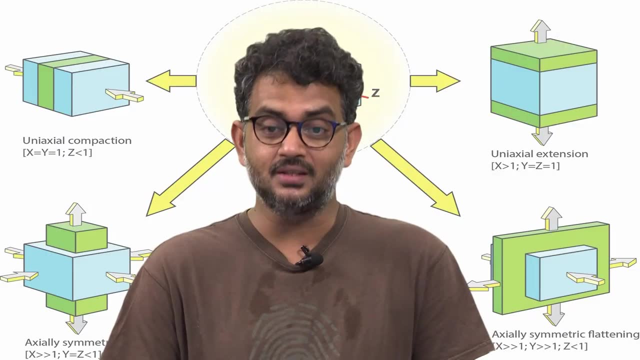 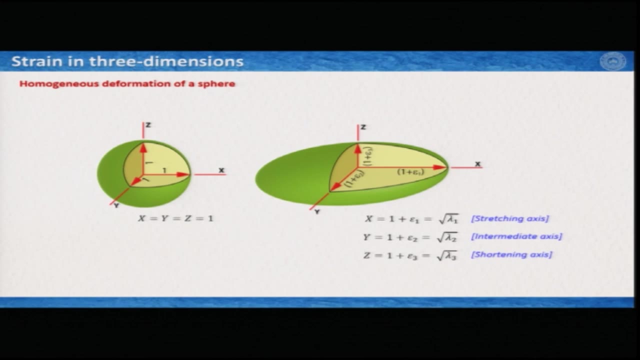 to 1 plus epsilon 1 and z equal to 1 plus epsilon 3.. Now let us have a look of what do we mean by strain ellipsoid, which is a transformation from a sphere. So if we deform a sphere homogeneously, then ideally it should take a shape of an. 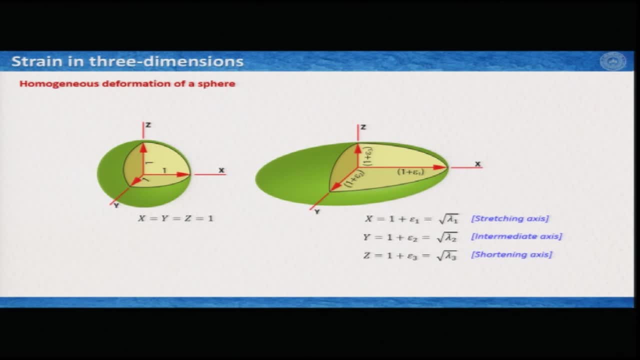 ellipse. So what do we see here? this is a sphere, and if we cut it perpendicularly from the middle, then we can get the 3 radii of the sphere. In this case, all these are unit. so this is 1,, this is 1 and this is 1,. therefore, this is undeformed, and x, y, z are all equal. 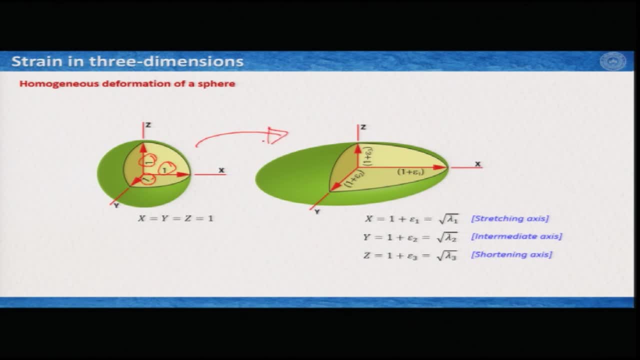 to 1.. If it transform to an ellipse due to homogeneous deformation, then this x, y and Z would change and therefore their values would change as well, and the sphere would take a form of an ellipse. In that case, Z would be 1 plus epsilon 3, X would be 1 plus. 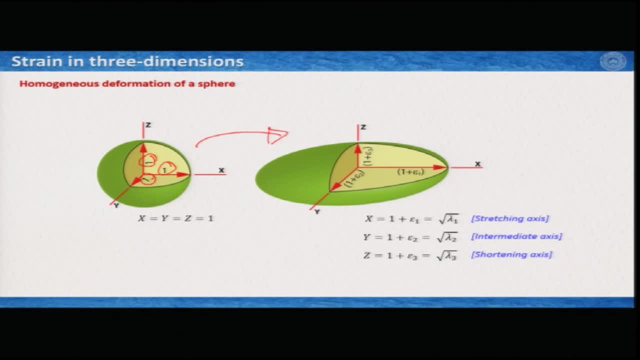 epsilon 1 and Y would be 1 plus epsilon 2 and therefore, at least from this visualization, as X has elongated most. that is our considerations. so X is the stretching axis, Y is the intermediate one compared to Z. so Y is the intermediate axis and Z which got compressed most. so therefore, 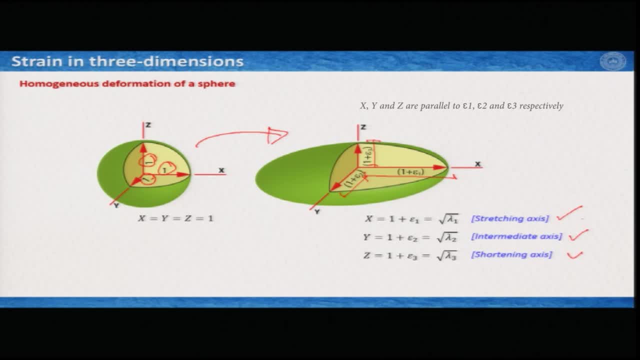 Z is the shortening axis. So these X Y Z, these three play a very important role, their deformations, their shortening, their extension relative to other two. Now, based on these relative elongations or relative shortenings of X Y Z, we can actually: 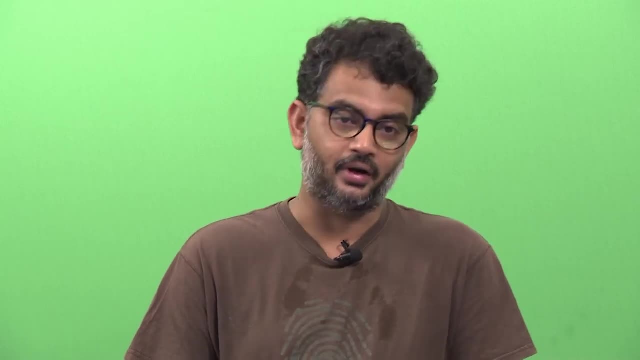 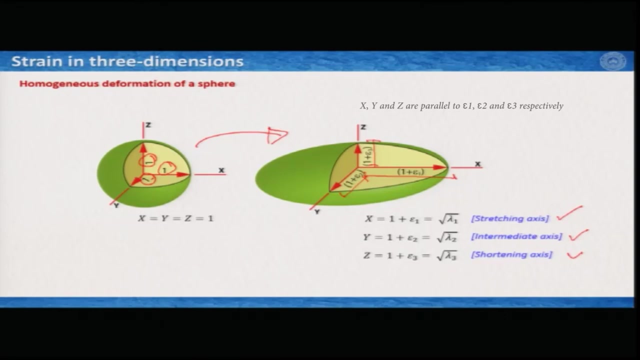 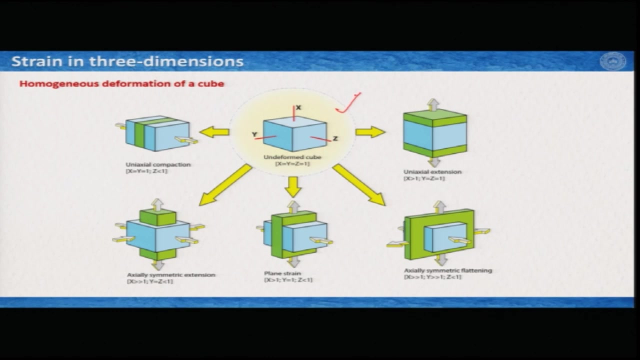 describe a number of possibilities or end members of strain ellipsoids, but this time, instead of ellipses we would look with an unit cube. So what we see in this diagram, this is the unit cube, highlighted by a circle where X is vertical, Y and Z are oriented horizontally. this is undeformed cube, therefore X, Y, Z. 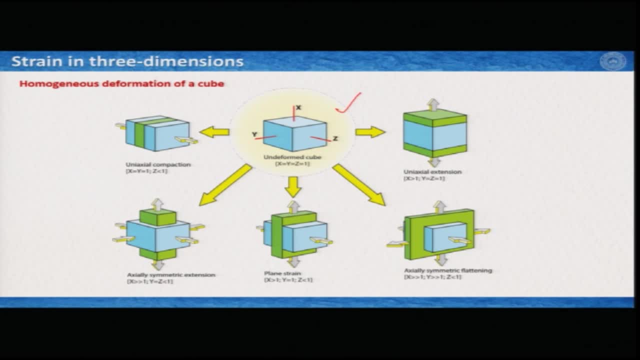 equal to 1.. Now one can deform this cube in many different ways, but here what is shown by this 5 illustrations at this 5 sides, these are the some sort of end members of the deformation in three dimensions. The first one we will take over is uniaxial compression or compaction. so before I go, 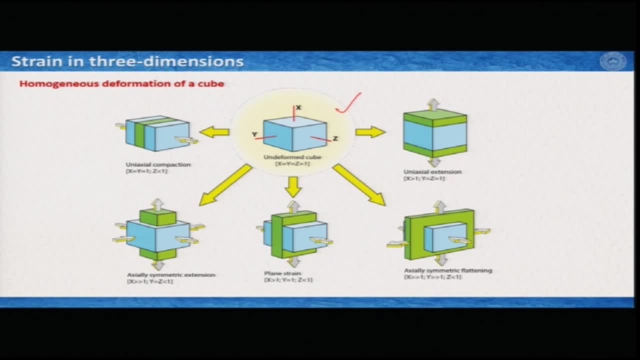 to this. go to the description of this deformation. As you see, this blue cube is the undeformed cube and what we see in the green colors these are deformed shape or from the cube it got transformed to the shape of this, and these are all in three dimensions. 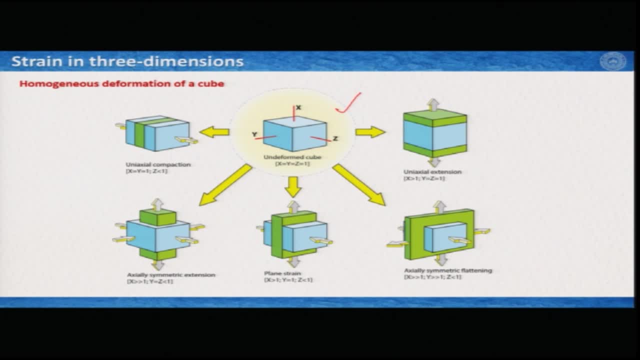 So what do you see here? uniaxial compaction, as Z is the shortening axis, so the compaction happened along Z. X and Y remain, remain same, as you can see. this is the x direction, So x is constant. this is the y direction. 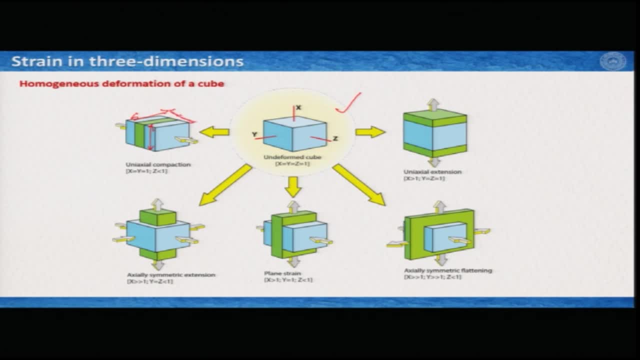 y is constant, but z. instead of this length, it is now got shortened. and it got shortened in one direction, along one axis, z axis. So therefore, this is uniaxial compaction. Now, in this side you can also do uniaxial extension. in that case x is the maximum stretching. 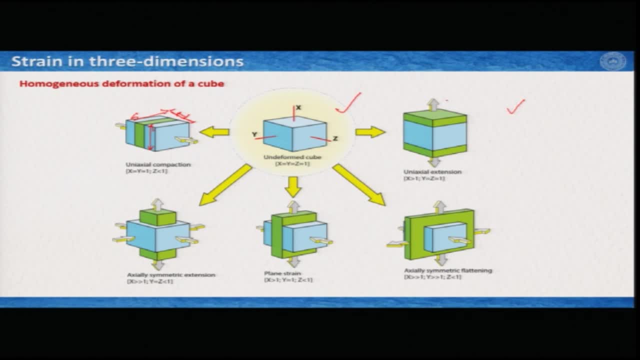 direction. So extension should happen along the x direction. So this was your initial length along x, but now it got changed to this magnitude, whereas z and y remained same. Therefore, this is uniaxial extension. Now there are three other possibilities. one is: 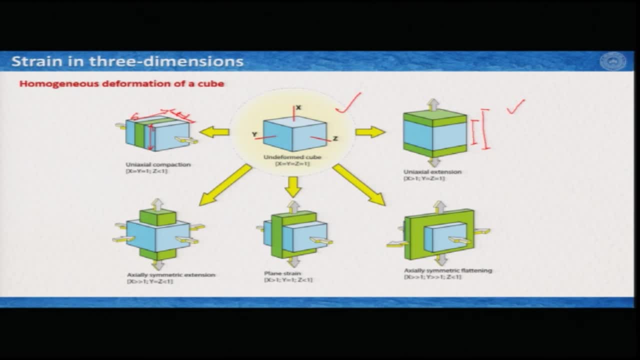 axially symmetric extension. that means it gets extended in one direction and shortened in in other two directions. So therefore it got extended along x direction but got shortened along y and along z direction. The other possibility is plane strain. this is a very important 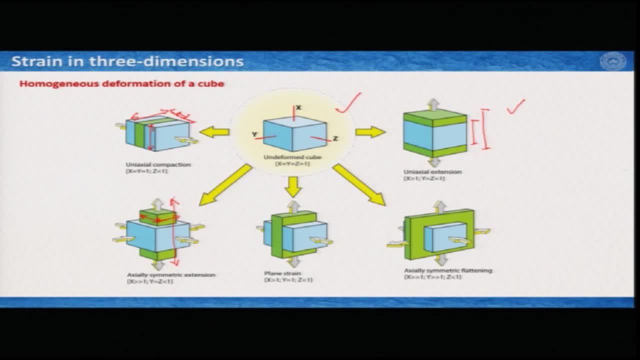 term that you need to learn. Plane strain is when in one direction there is no strain, but in other directions, yes, In this case, this illustration, what we see here: this unit cube got extended along x direction. it got shortened along z direction, but its y direction. 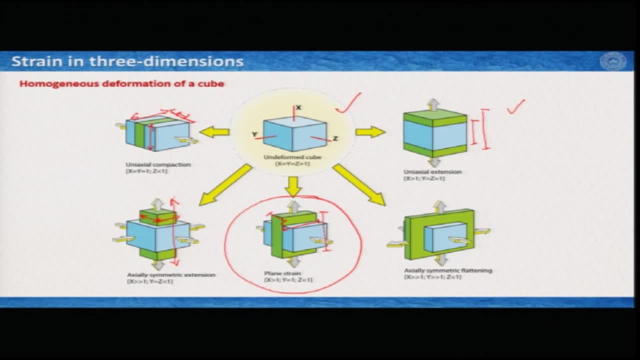 remained constant length as it was. So therefore it is plane strain, that is, along one direction there is no strain, And the final one is axially symmetric flattening. What happens in this case? that only one axis shortened very much and other two axis they extend highly. So what we see here, as you, 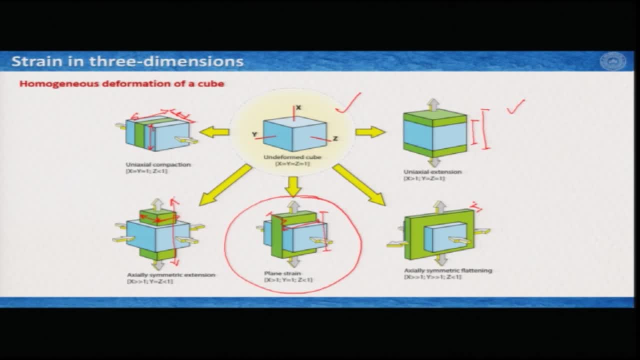 can see the z direction. it got highly shortened and this is the x and y both. this is y and this is x. They both got extended along x direction but it got shortened along z direction. but they both got extended significantly compared to z and this is known as axially symmetric. 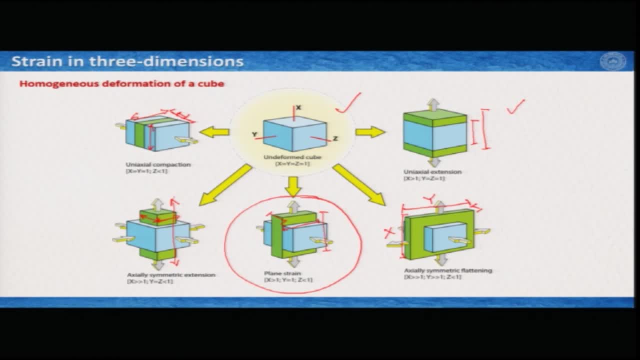 flattening. Now, before we switch to the next slide, there are many books or many texts or many web materials. you may find this: x, y and z, these are oriented different ways. So you may find that x and y- these are placed horizontally and z is vertical. We may use, in some cases, we may 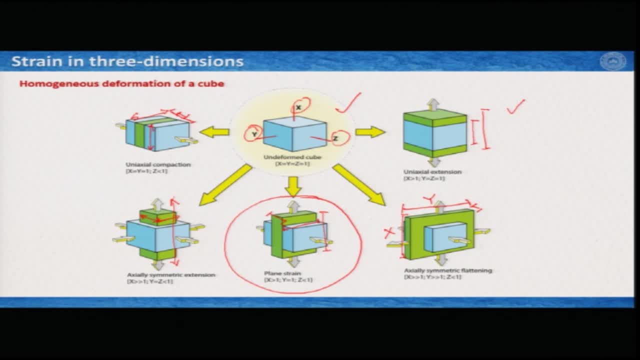 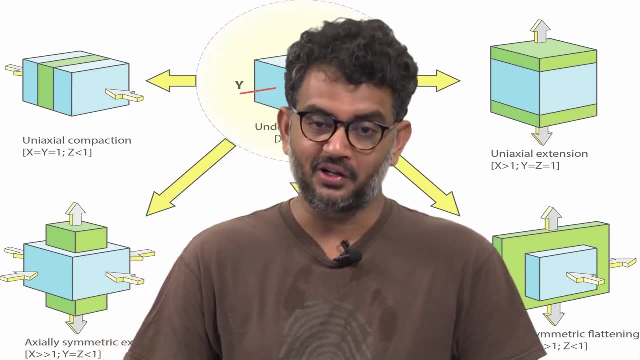 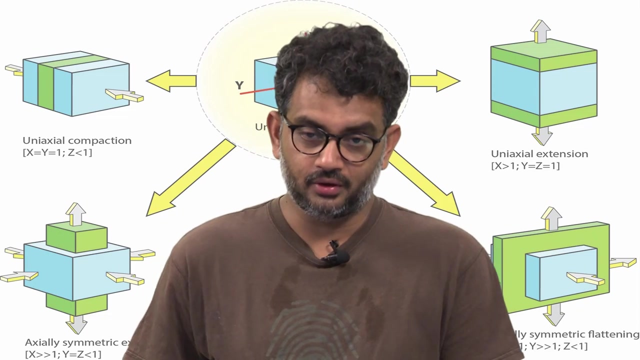 use these illustrations as well, but whenever you look at such diagrams, it is very important that you first make sure you know where is your x, where is your y and where is your z compared to the deformation pattern Now, based on this idea of deformation of an undeformed. 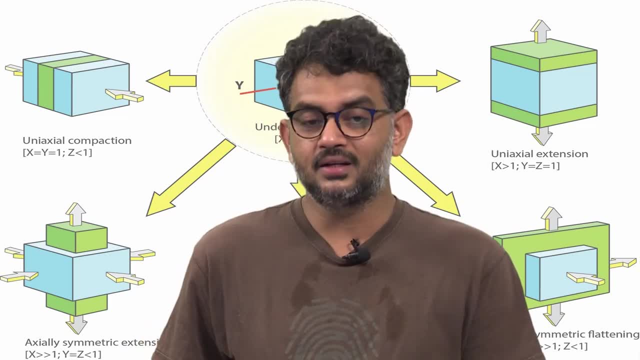 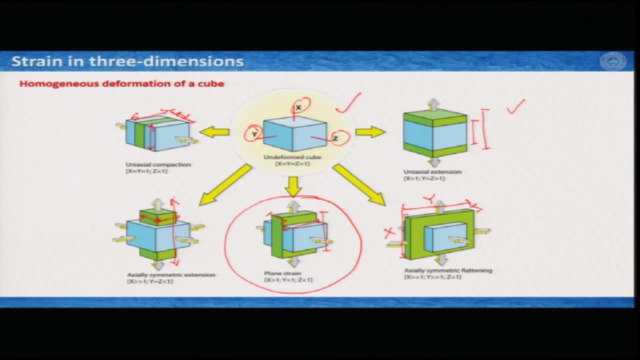 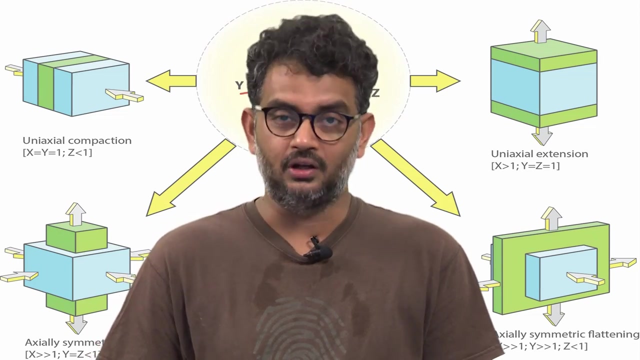 cube to these different possibilities. you can understand that once these materials, they do deform In different ways, you would produce different types of strains. that means the rocks would deform differently. and at the same time, because the rocks would be deforming differently, you will see different types of features in your rocks, and we will see this now. So the 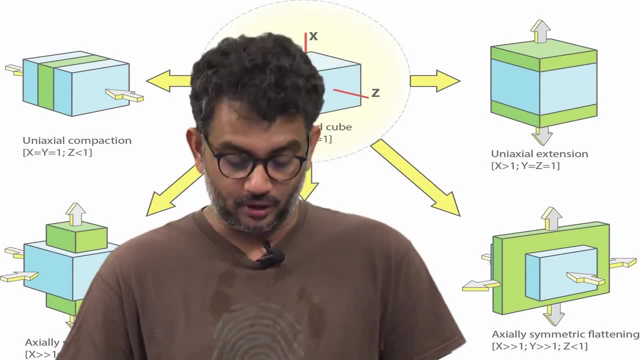 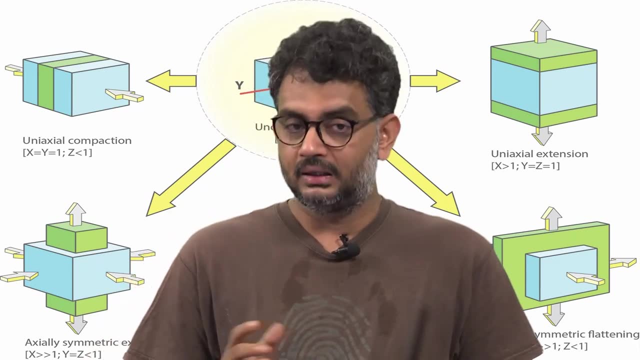 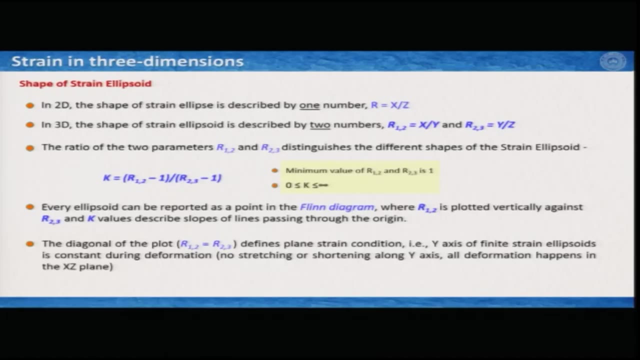 best way to explain these different types of deformation is known as Flynn diagram, the description of three-dimensional strain ellipsoid. The strain ellipsoid is best represented in Flynn diagram, So in two dimensions. the shape of the strain ellipse that we have described by only one number. if you remember, that was. 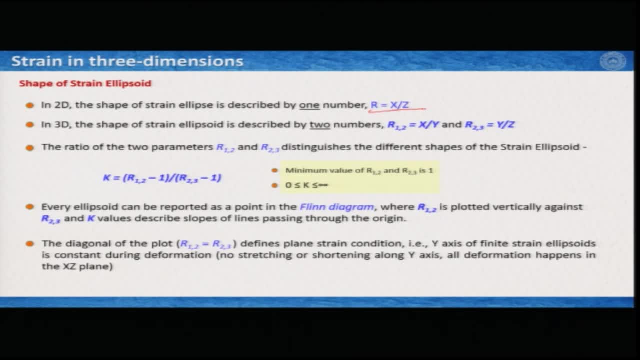 r, which was the ratio of long axis versus short axis, But in three dimensions. the shape of the strain ellipsoid is described by two numbers: One is r12, which is the strain ellipsoid. The strain ellipsoid is the strain ellipsoid. 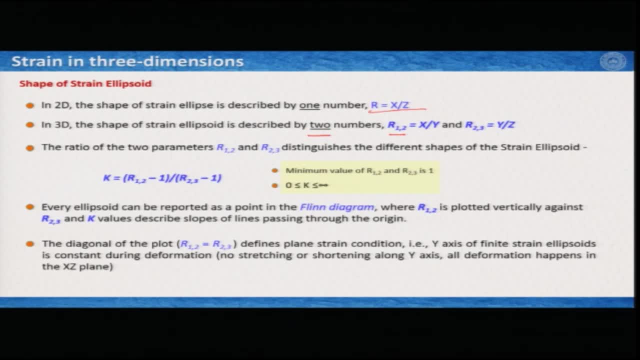 is the ratio of long axis versus intermediate axis, and another one is r23, which is the ratio of intermediate axis versus short axis. Now, the ratio of these two parameters, that is, a ratio of r12 and r23, describes and distinguishes the different shapes of the strain ellipsoid. 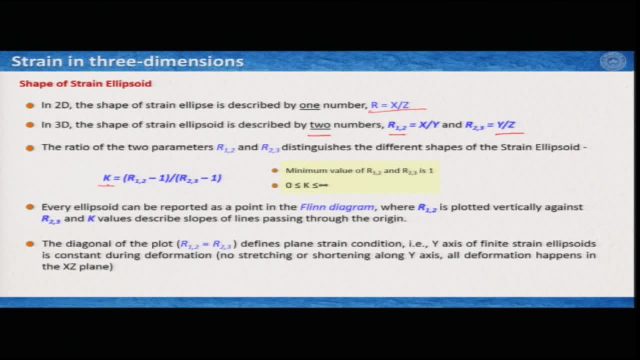 and this number is known as the series variable. So you get that this story and this information is also which you find in the minute form, Though the sequence is the series variable and has k, where k is defined as r12 minus 1 divided by r23 minus 1.. So, from this equation and 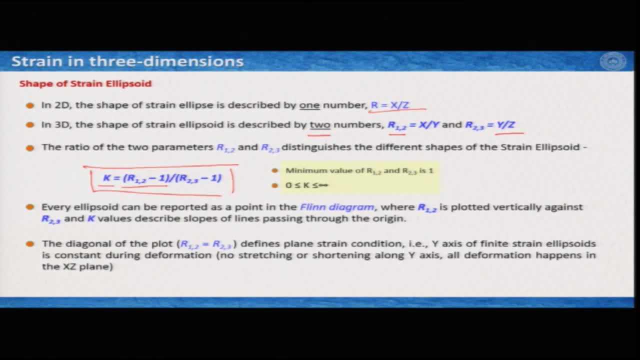 our understanding on x, y, z, we can figure out that minimum values of r12 and r23 possible is 1 and k can be from or could be equal or greater than 0, and equal or greater less than infinity. Now, given this condition that k could be 0 to infinity, so you can report. 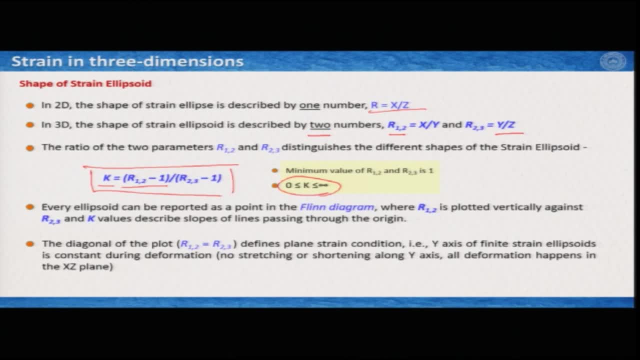 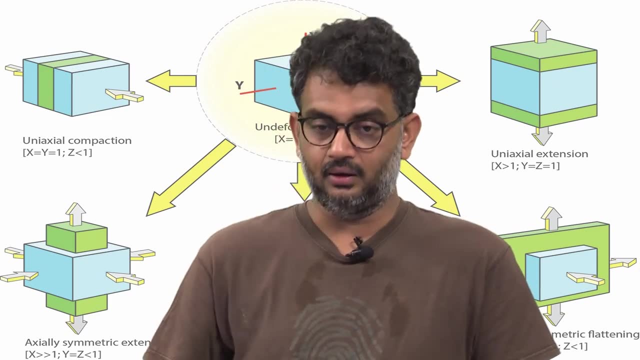 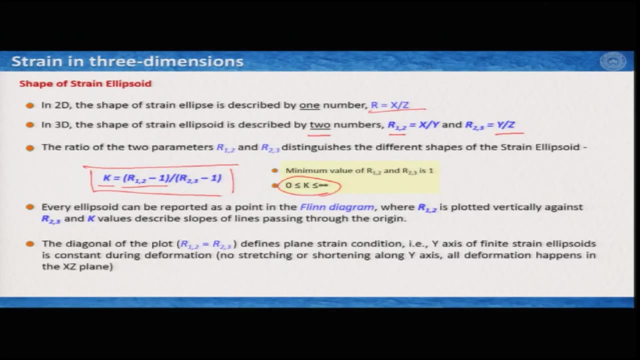 the all possibilities of strain ellipsoids in the Flynn diagram, and the Flynn diagram we will see in the next slide. It is actually sort of a two-dimensional Cartesian plot where x axis is represented by r23 and y axis is represented by r12 and you can plot a number of k values in between. So the diagonal. 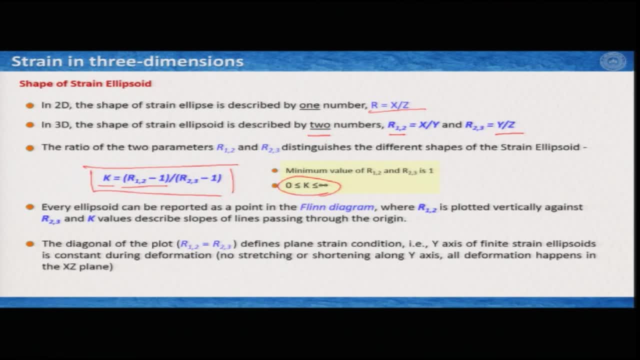 of this plot, as we will see soon. that is where r12, equal to r23, is actually defining the plane strain condition, That is, y axis of the finite strain. ellipsoid is constant during the deformation. That means we have learnt it before, that there is no stretching or no shortening along the y axis. 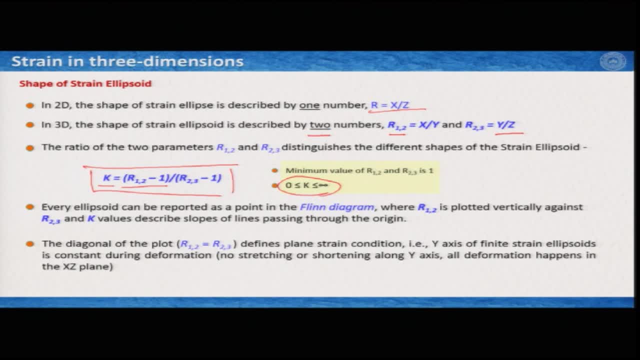 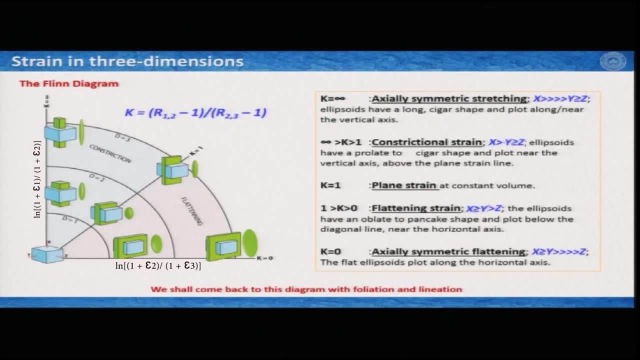 Whatever deformation happens, that happens along the x and z axis and therefore on the x- z plane. So this is the Flynn diagram we are talking about. As you can see, this is the plane strain of the finite strain ellipsoid. Now let us see that along the x axis we 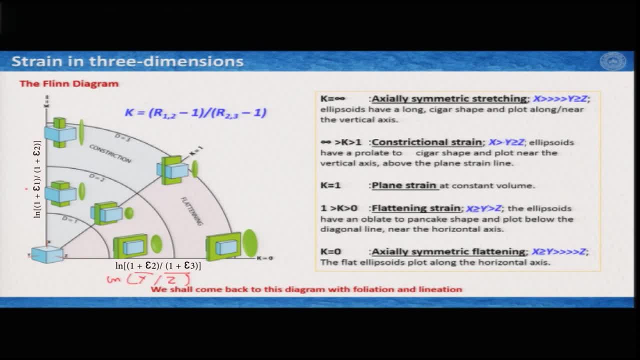 have plotted this and in this case this is again long axis, which is x, and here this is y, and again, all these things are under log. Now this log is used to accommodate different shapes or sizes of the measurements, so different magnitudes of the measurement, if you have a high value and if you have a small value. 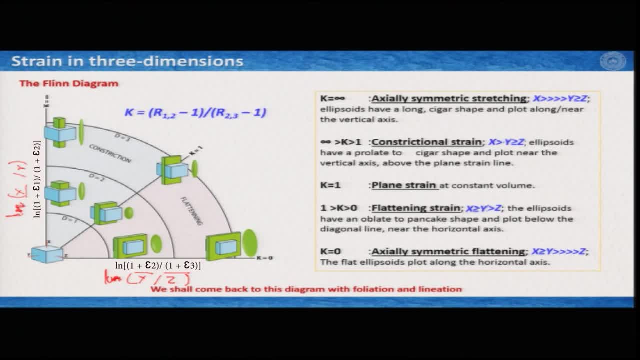 of the measurements, then you can plot everything in the same diagram. Let us try to understand this diagram in detail. So, as we said that along this line, which is running 45 degrees with respect to this x and y axis, this is where k equal to 1 and. 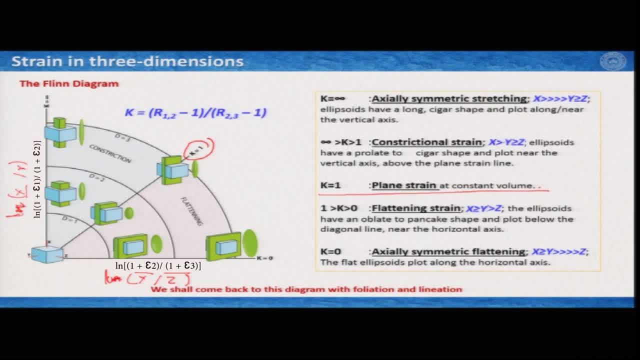 as we have said, k equal to 1, you have plane strain at constant volume, As you can see here. at this magnitude of strain, the y axis remained constant. even I increase the strain, magnitude y axis remain constant, but it extends along x and shortens along z direction. So 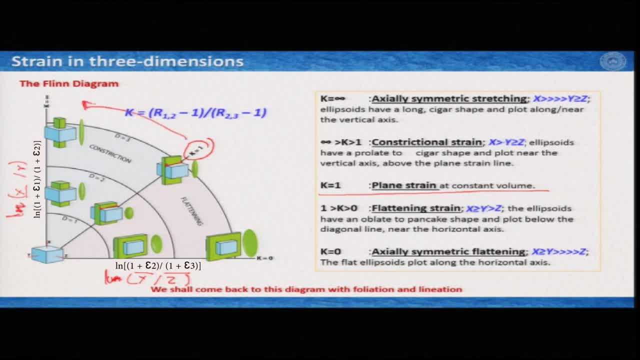 whatever left on both sides of this k1 value if I go to the top side that says that it is is under the constriction domain. that means that in this domain everything would deform. I mean, I am sorry, along x axis it would extend and other two directions it would shrink. therefore, 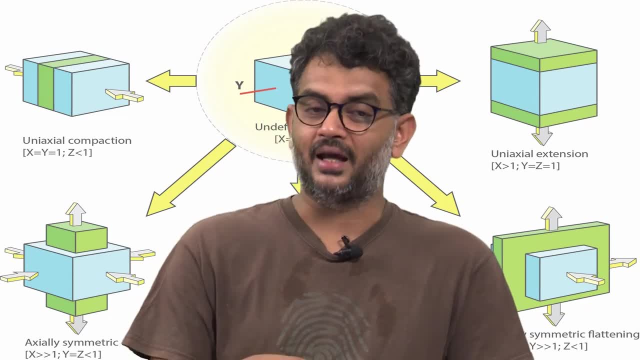 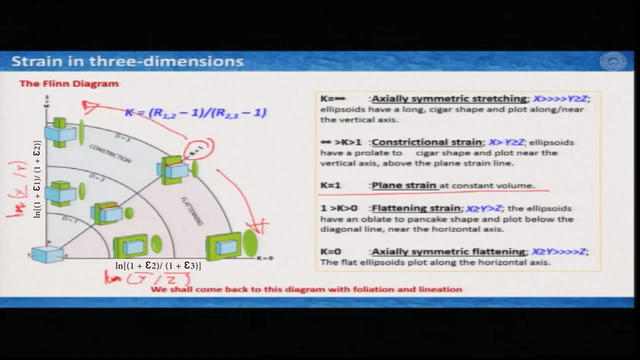 with progressive deformation, you would produce something which is like a pencil or like a long object. On the other hand, if we go to the flattening side, which is the downside of this k equal to 1 direction, there the deformation would happen in axially symmetric manner, or. 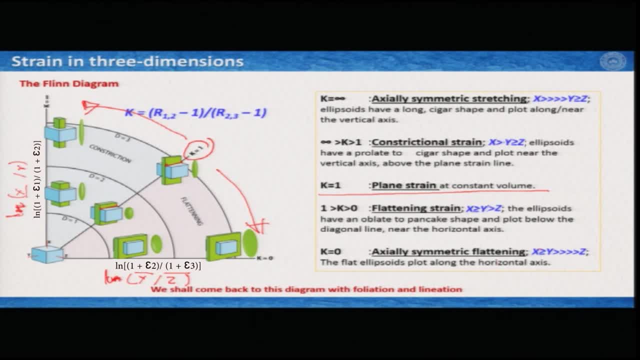 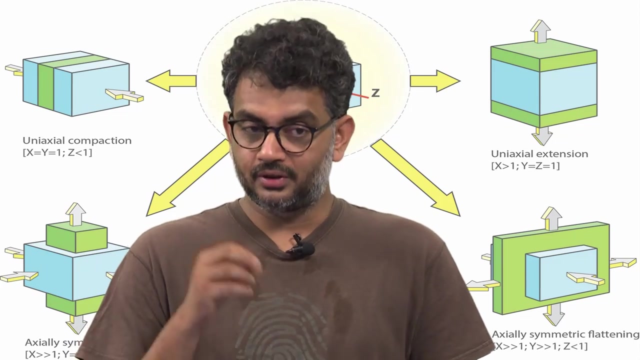 axially symmetric flattening manner where x is greater than or equal to y, and this x, y values are much greater than z. Therefore you would produce something like a pancake or like a flattened disk. So if I go towards this side- k equal to infinity, then I produce rocks, characteristically with some sort of. 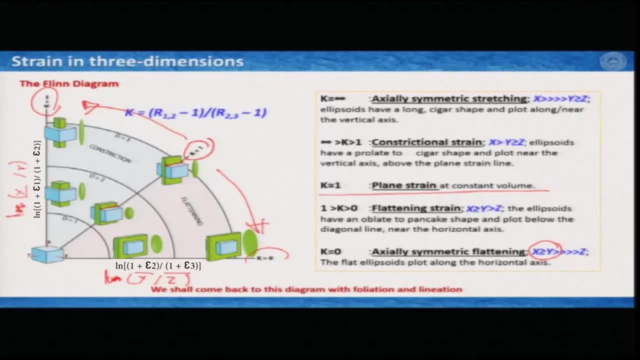 linear features and if I come to this side, k equal to 0, the deformed rock would show a lot of flattened objects. Now, considering this idea, you can figure out if I am in the constriction domain. then the rocks would tend to produce more linear features through deformation. and at k equal 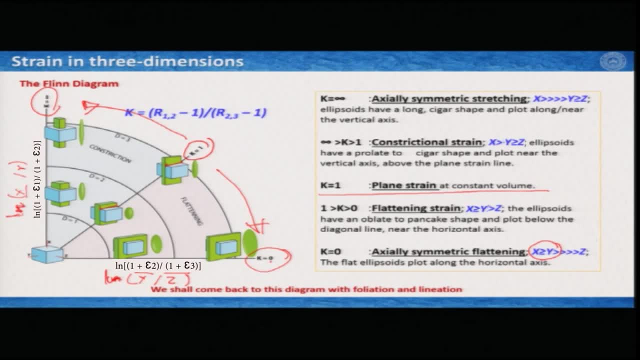 to 0. the rocks would tend to produce more flattened or planer fabrics. Therefore, this rock shear would be prone with the caustic caused deformation. In other words, thisyet hot on withformed ones will produce more linear features because there will be only riff ideas. 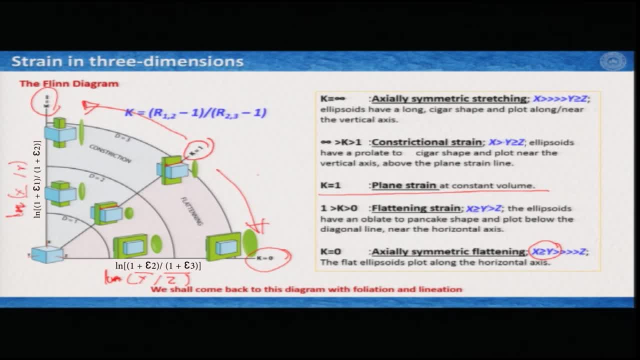 velocity and therefore k equal to 0 or, in this domain, whatever we produce towards this side, we call it S-tectonites and here, because we will be producing lineations dominantly, these are known as L-tectonites, and whatever stays in the middle it would have both lineations. 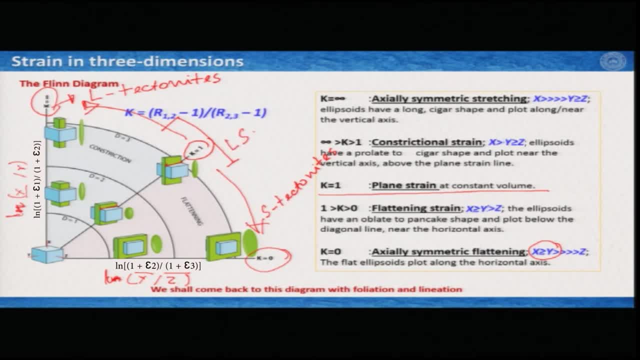 and schistosity. therefore these are known as L-S-tectonites. We learn more about L-tectonites, L-S-tectonites and S-tectonites when we will study foliation techniques And lineation in one of the next lectures. so we will come back to this Flynn diagram. 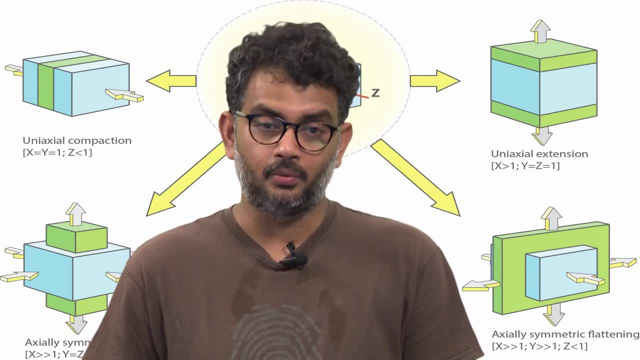 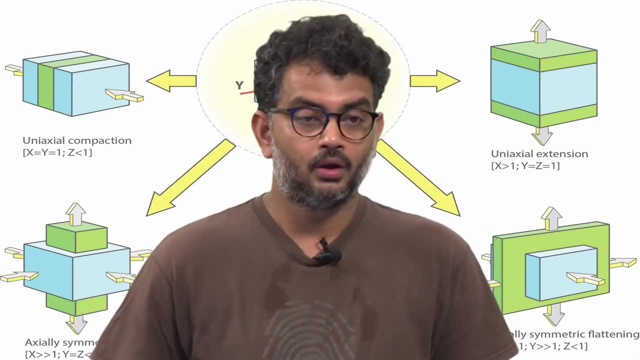 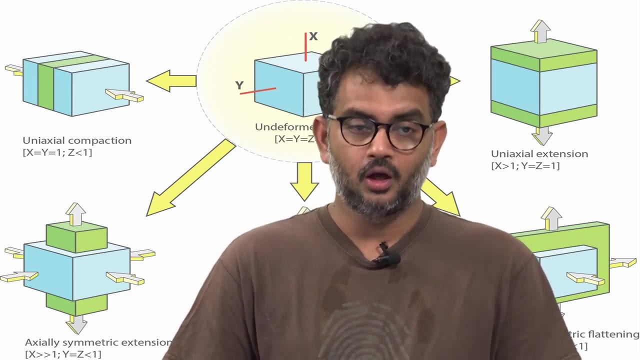 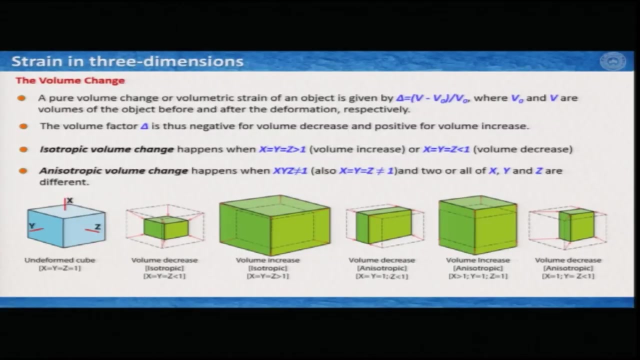 again and again for more interpretation of deformed rocks. Now let us talk about the volume change. so we have discussed so far its homogeneous deformation without volume change. but volume change, like it happens in two dimensions, it can also happen in three dimensions. So pure volume change. 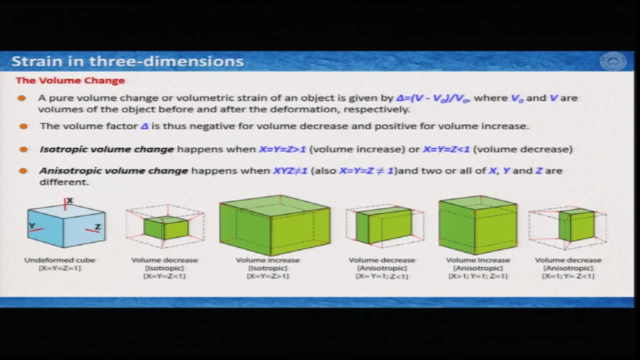 Or volumetric strain of an object, as we. it is a very similar equation that we have seen. so it is a ratio of the change of the volume with respect to the initial volume. So you can say that volume change. or if you say this is delta, then it is defined as V-V0. 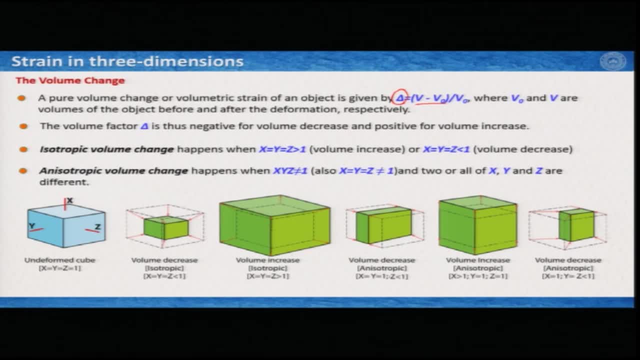 by V0.. Where V0 and V are volumes of the object, So V0 and V are volumes of the object. So V0 and V are volumes of the object, So V0 and V are volumes of the object. 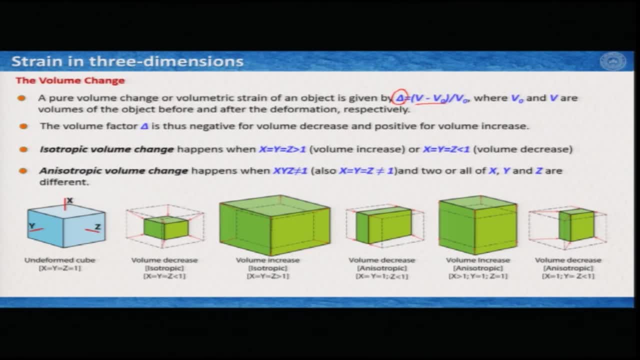 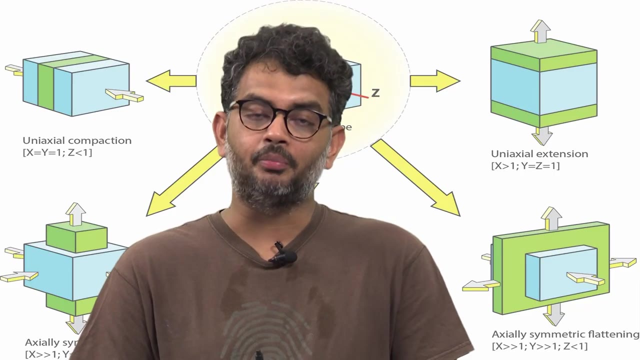 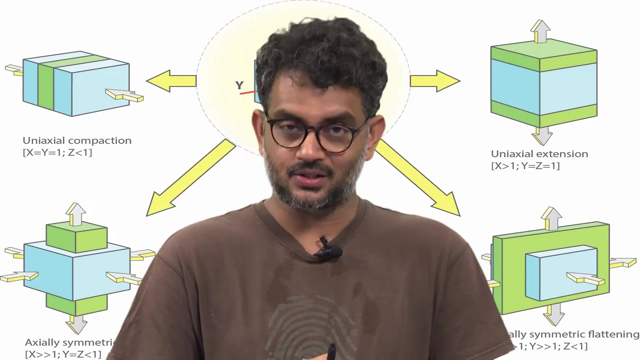 Before and after the deformation respectively. So the volume factor delta is thus negative for volume decrease and positive for volume increase. Now volume decrease and increase. whatever happens, it can happen either isotropically or anisotropically. If it happens, isotropically means that all principal axis of strain are either extending, 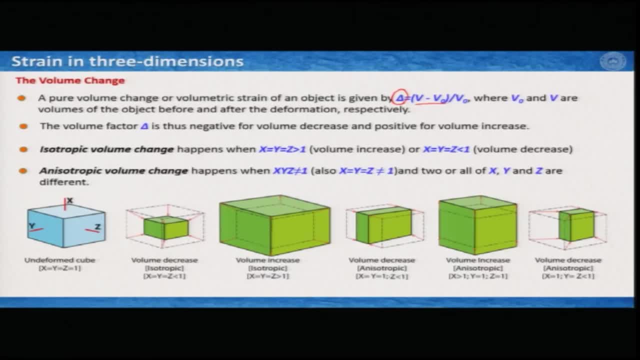 or shortening equally. And if that does not happen, then it is anisotropic volume change. So isotropic volume change therefore could happen when x, y, z, they are all greater than they are all equal and greater than equal, greater than 1, therefore you would have volume. 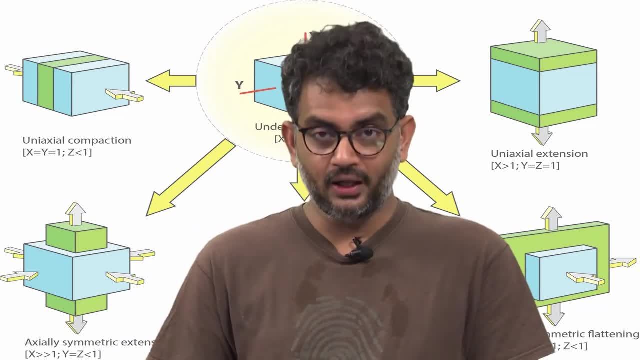 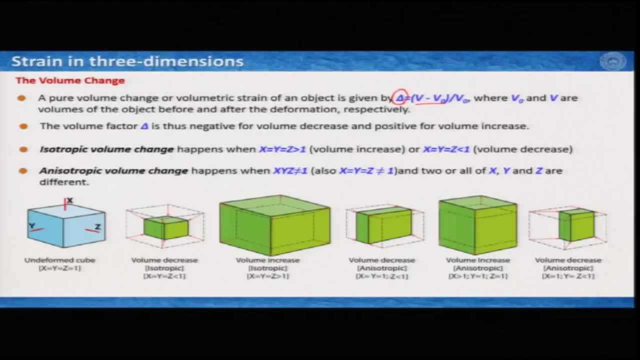 increase, and if these are all equal but the values are less than 1, then you have volume decrease. So here I have tried to show this with some illustrations. So again we have this undeformed cubes, undeformed cube here you have x, you have y, you have z direction. 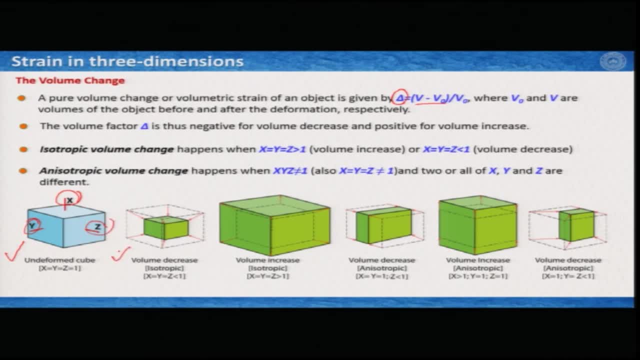 here, as you can see, in the first illustration, where volume has decreased isotropically all these directions, the shortening was equal. along all these directions, the shortenings were equal. In the second diagram, where the volume has increased, again along all directions, the extensions or elongations are equal. 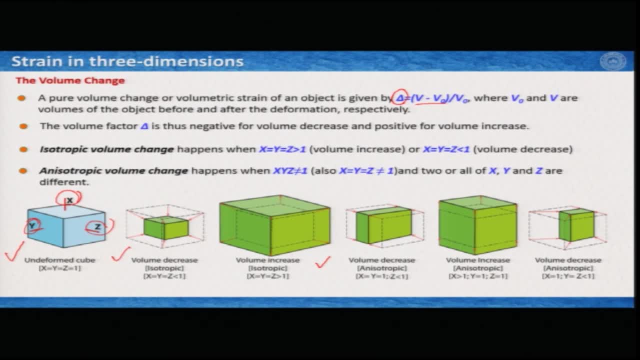 Now anisotropic volume decrease essentially where your x, y, z would not remain of same values, So they could be either greater than 1 or less than 1. they could be equal to 1 or not equal to 1, does not matter, but they cannot be equal to each other. 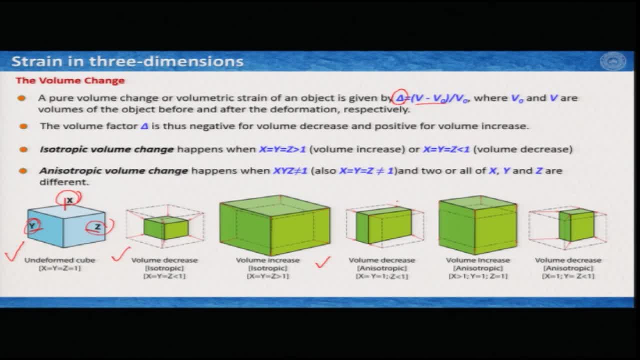 So here there are three examples. So in the first case, what we see? that volume has decreased anisotropically, where x and y did not change. So therefore, your x remains constant, y remains constant, but along z it decreased its volume. 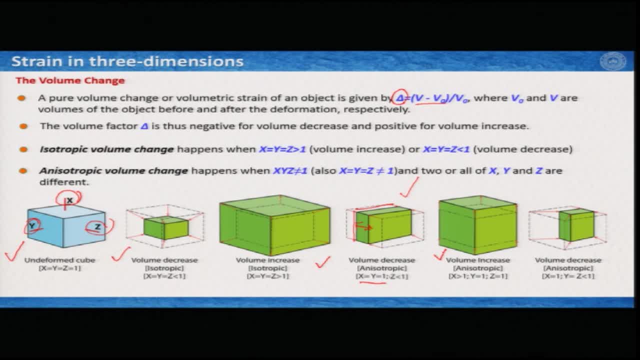 In this case the second example, which is also anisotropic volume increase, but in this case x has extended, but y and z. this is your y and this is your z. Sorry, This is y, this is z and this is your x. so you can see, x has extended, but y and z they. 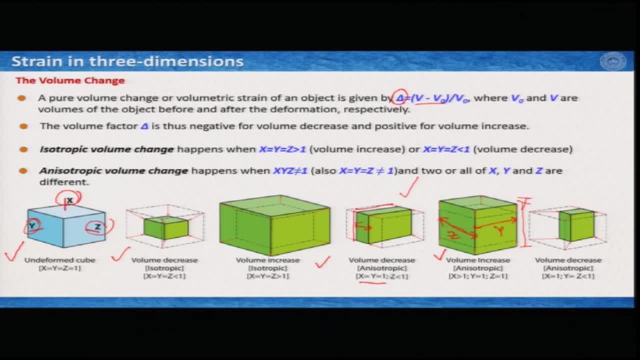 remain constant. So therefore, volume has increased, but anisotropically. and in the third and final example, what we see here, volume has decreased, again anisotropically, where nothing has changed along the x direction, but it got shortened along y direction and also it got shortened along z direction. 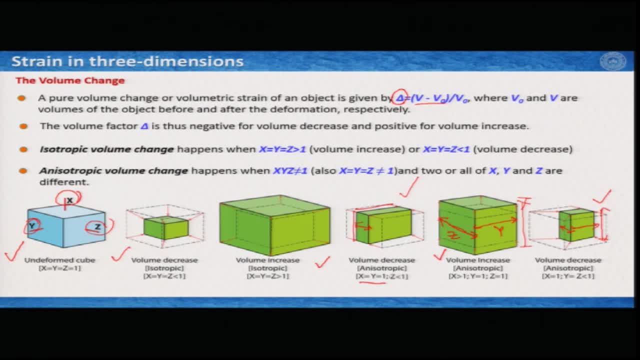 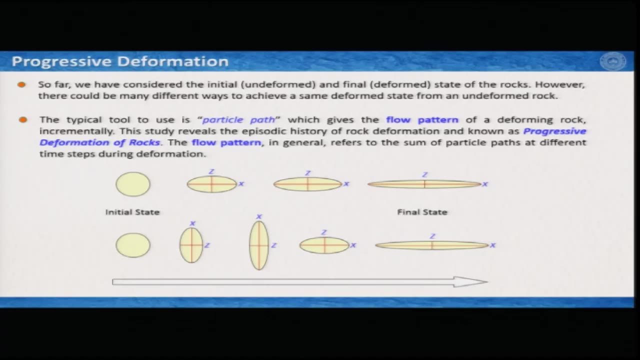 Now. so we have learnt so far that homogeneous deformation in three dimension and also volume deformation. that means you can change your volume in three dimension as well. The next topic we will discuss in this lecture is progressive deformation. Now, if you remember the first lecture of strain, we talked about initial position finalization. 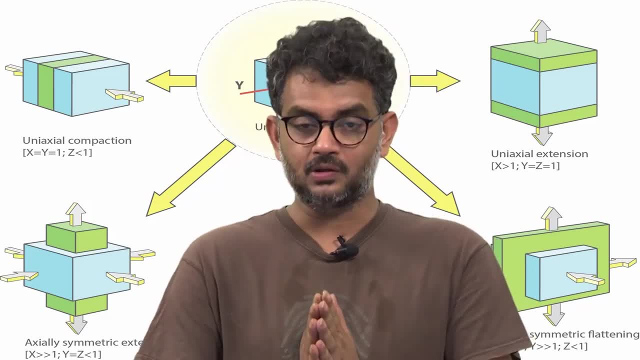 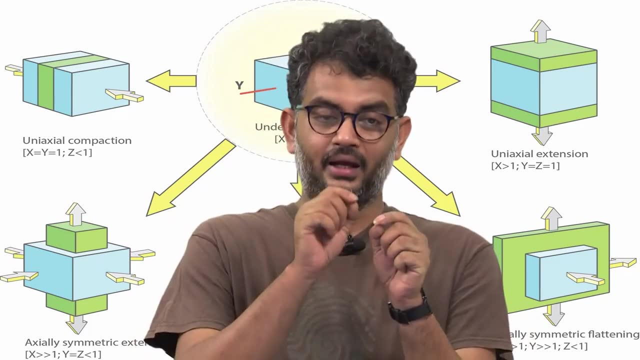 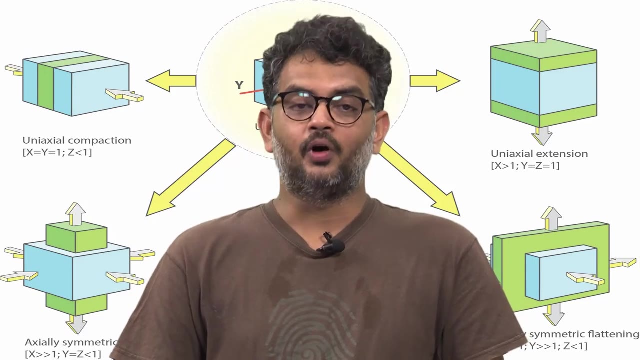 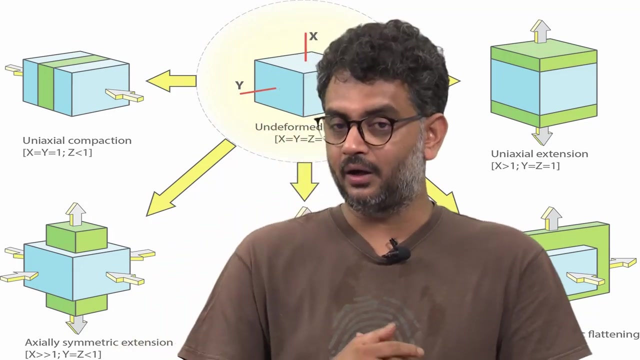 final position and in one set of examples we talked about displacement vectors, where we connected the initial position with the final position and added these two points by an arrow, and from initial to final position we added the arrow heads and that was a vector, But then there was also another column. 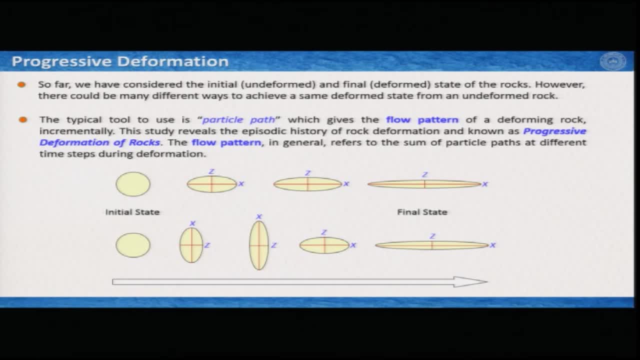 was particle path where we actually could track that, how this point was moving from its initial position to the next position or to the final position And depending on whether you are doing rigid body rotation or translation or deforming the material by simple shear, pure shear or any other ways we can see or we can understand. 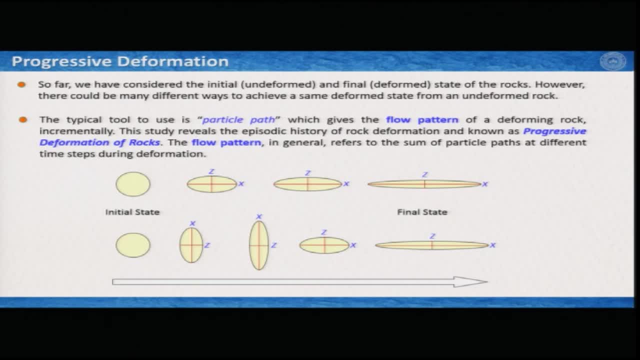 that this displacement vectors are not necessarily equal or they are not necessarily similar to those of the particle paths. Now the study of this. particle paths actually fall in the domain of progressive deformation, So there could be many different ways to achieve the same deformed state. that is the point. What we see here. we have initial state in these. 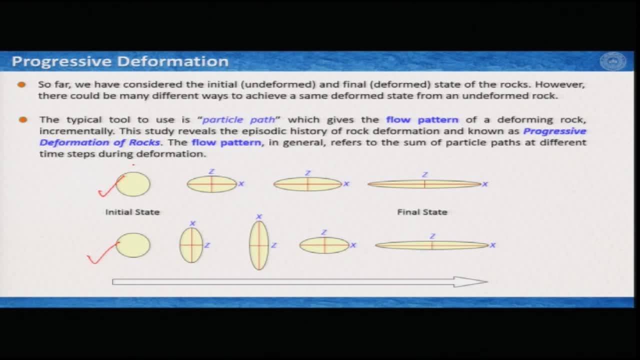 two rows, Both are circles and the final stage, both got into dimension. we are looking at and we got a strain ellipse. Now what we see here, from here to here, if we look directly then they look similar. So the displacement vectors, if we try to draw from this position to this, 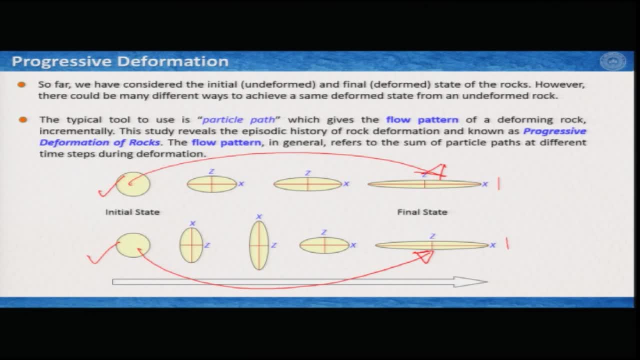 position. in both cases it would be similar. So the displacement vectors, if we try to draw from this position to this position, in both cases it would be similar, but in between there could be many different possibilities. So the first example is very straight forward, that I had a circle, then little more strain. 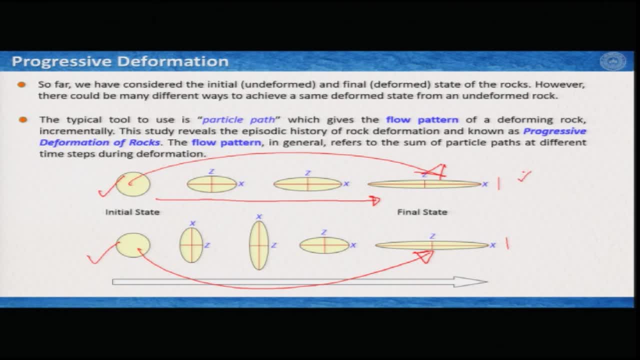 even more strain and further more strain. I achieved to this state, But in the second row, what we see, that it took a different shape, it deformed differently from here to here, from here to here, from here to here and finally we could reach here. So displacement vectors. 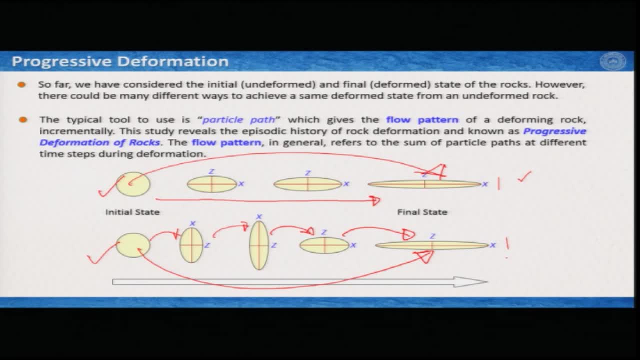 here in these two cases would be very much similar, but not the particle paths and again, this study is progressive deformation. So in the next three slides we will have a look that what could be the possibilities or what could be the characteristic particle paths or flow patterns of deforming rock in 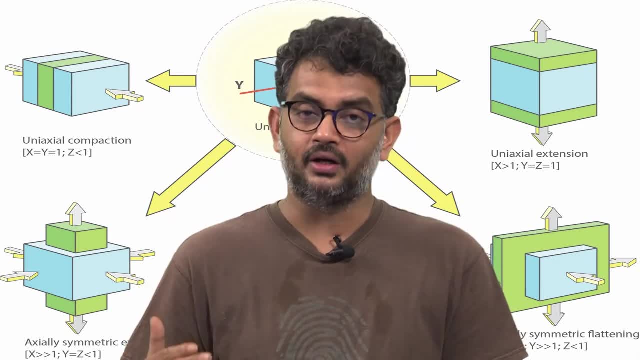 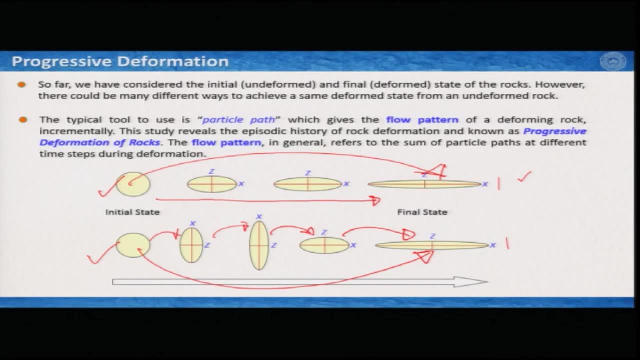 terms of pure shear, simple shear and the combination of these two. and before that, what is flow pattern? Now, flow pattern of a deforming rock is actually. it refers the sum of particle paths at different time steps during deformation. So it is: you add each and every particle. 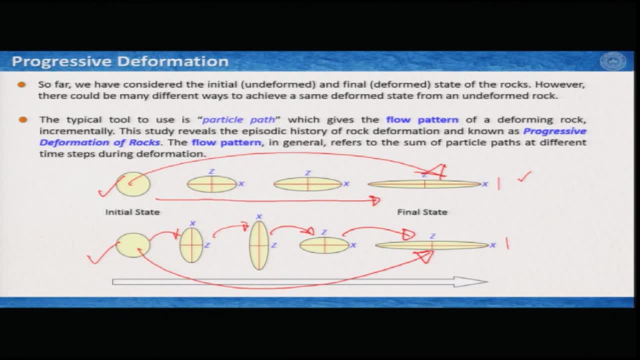 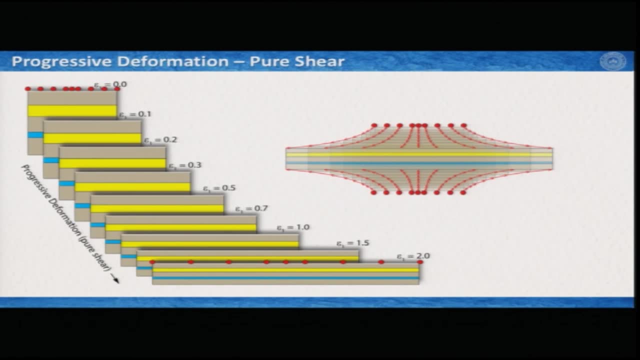 path and accumulate them. what you get is your characteristic flow pattern of a particular type of deformation. So what do you see in this slide, on the left slide? I particularly would request you to focus in this side that here I had in two dimension, I had a square. 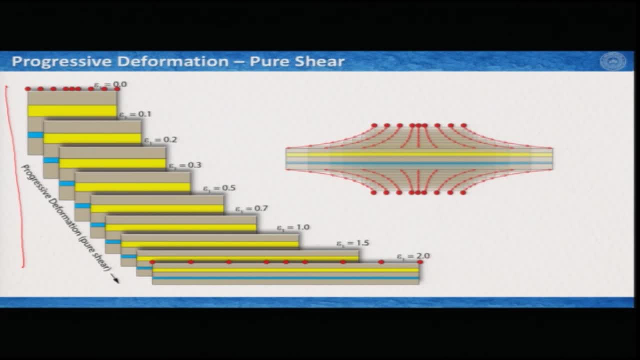 and then progressively, I deform this square to achieve a finite elongation or finite deformation along x direction of 2.. Of course you do not see the individual squares and later rectangles, just because I had to fit them in a single slide, But they are cascaded in this way, So the strain progressed this way. So first one: 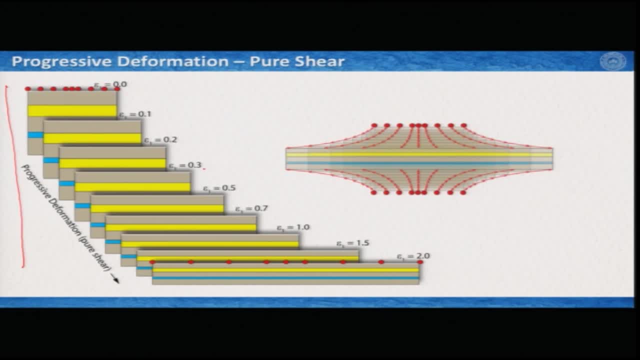 it is undeformed, and then slowly 0.1, 0.2,, 0.3,, 0.5,, 0.7,, 1, 1.5 and 2.. So this is how it progressively deformed, in a pure shear manner. Now, if I club them together, all these, 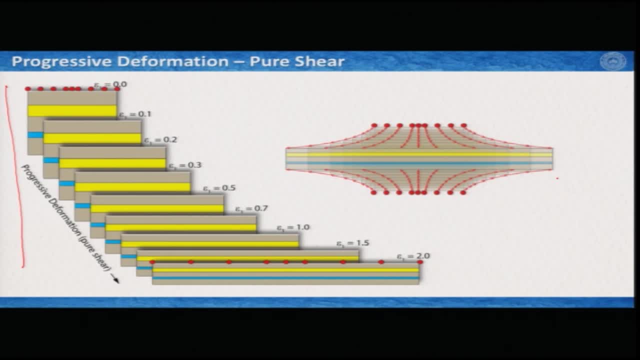 images, then they would appear something like that, and I try to track this little red line. So if I put these two red points in the form of particle paths, then this point would move to here and then so on. So characteristically, all these points, at least from the two sides. 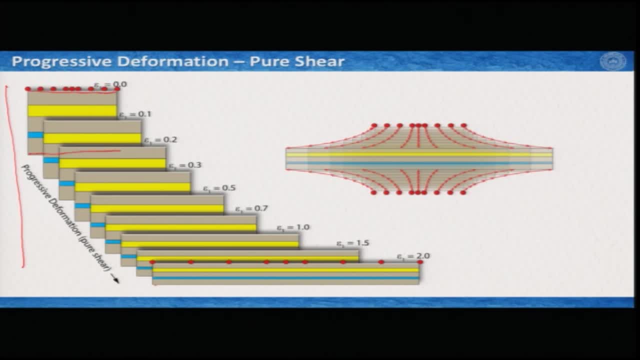 this top side and the bottom side and how they have arrived to their end. shape end- deformed shape. If we track the end of the deformed shape, what happens is that this point is at the end of the deformed shape. If we track this end of the deformed shape, what happens? 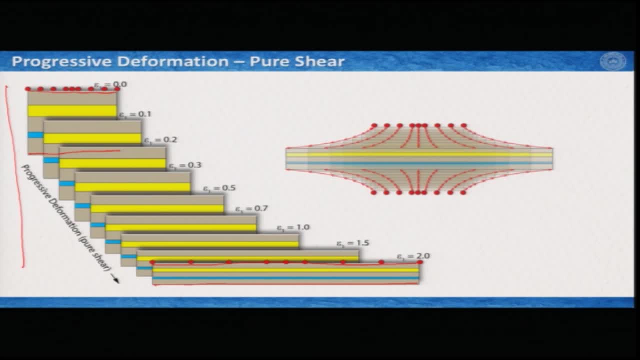 back each and every instances of deformation, then the characteristic flow path would be like this: what you see here in this diagram: by red arrows, So tiny red arrow heads, and finally you achieve a pattern. we will analyze this later. Now let us go to what happens if you have a simple shear deformation. again the plots. 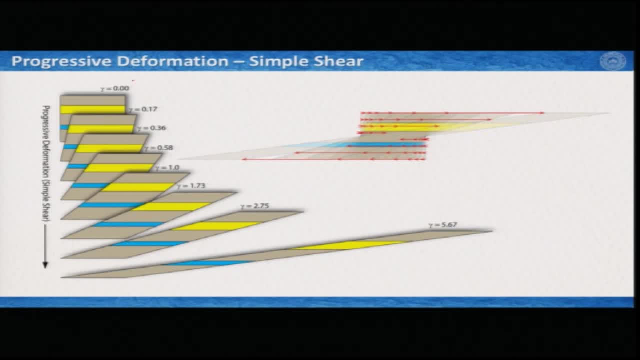 are in a very similar way. So I have a square and then I deform this square with progressive, simple shear. So here are the shear strain magnitudes given one after another, and again I can club them together as you can see here, and I see the particle paths or the flow patterns. 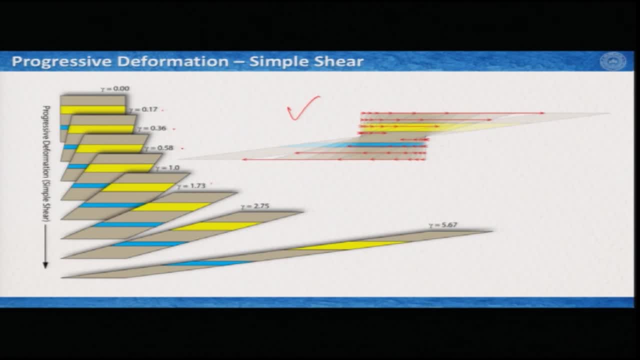 if I try to connect each and every point from one stage to the next stage, then it would be given as. So you can see here, with this red arrows in this side and this side, and what is interesting, that if you remember the previous slide, then it is characteristically different from pure 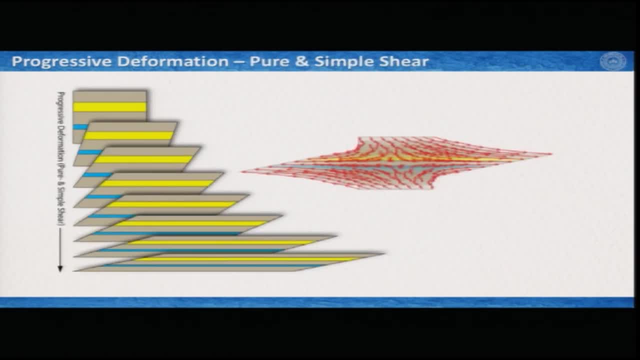 shear. Now, if we deform the same square, this square, in both pure shear or simple shear manner, That means I combine pure and simple shear, So you can see that I can combine pure and simple shear. So here again, in a similar way, we have the cascade of this rectangles. 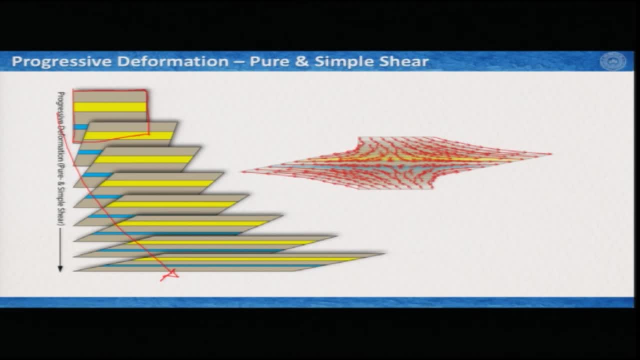 and then what we see here. again, if you club them and try to see the flow patterns, then it is extremely different. We see that these things are going this way, these things are going this way, and so on. So, again, this is very different to what we have seen with pure 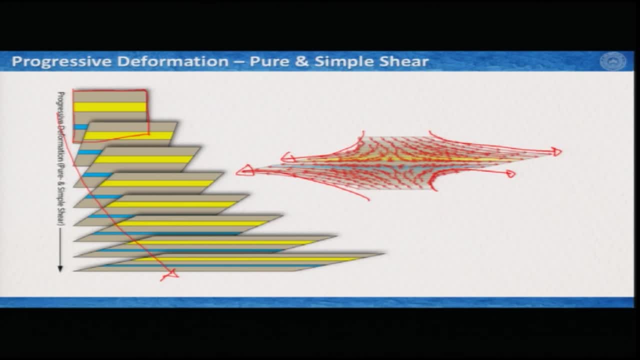 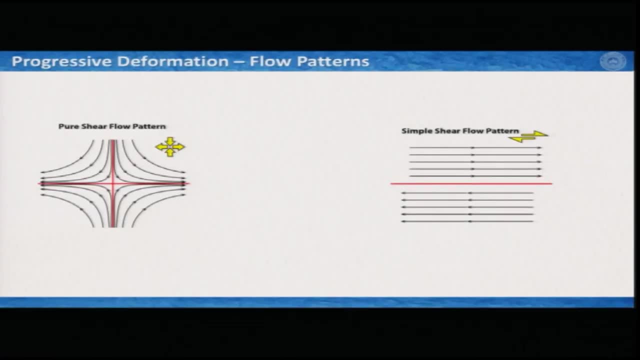 shear and simple shear separately. So what do these flow patterns tell us? Let us have a look. So if we see the pure shear, this is the simple form. These yellow arrowheads are showing that this is your compression direction and this is your extension direction in pure shear. 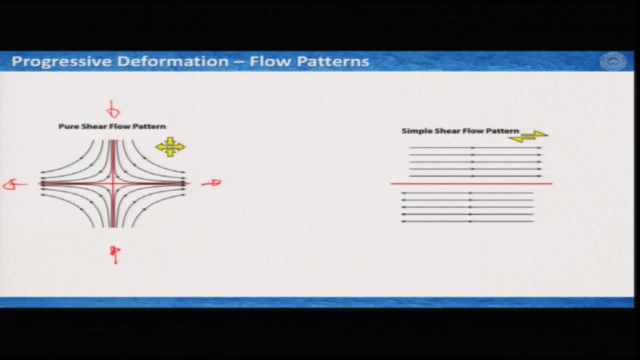 What we see here, That any material point here is moving and slowly changing. with the slowly it is going towards the extension direction and while doing so, initially this material line or points are in the compression domain. So in this direction they are in compression and similarly this is symmetric along the axis. these are your compression domain and 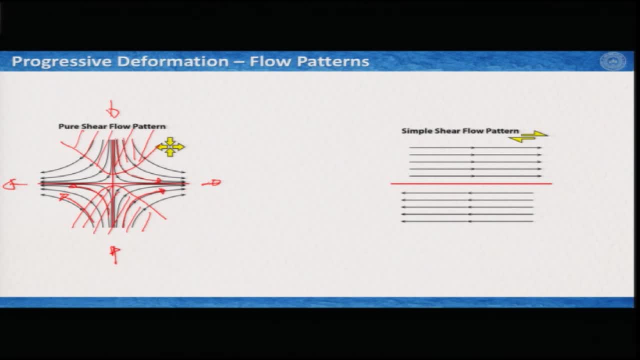 on the other side. this is your extension domain In simple shear. it is not so easy to apprehend the compression or extension looking at the flow pattern, but you can see the flow patterns are very much straight and they are moving opposite to other sides, other side of the. 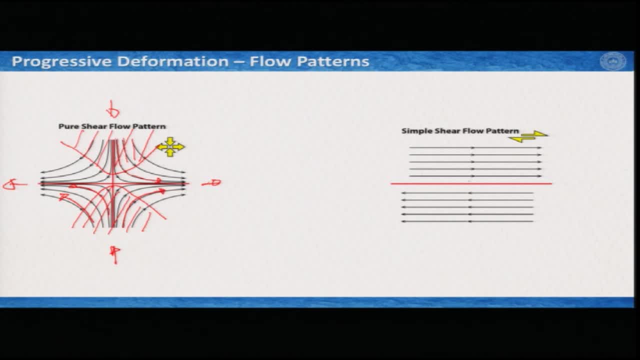 flow lines. Now, in this case, because if I had a circle here, the circle would deform to an ellipse of this And therefore I can assume that, or I can conclude that this would be my compression domain. that means, the compressions are coming from this direction and this would be my extensional. 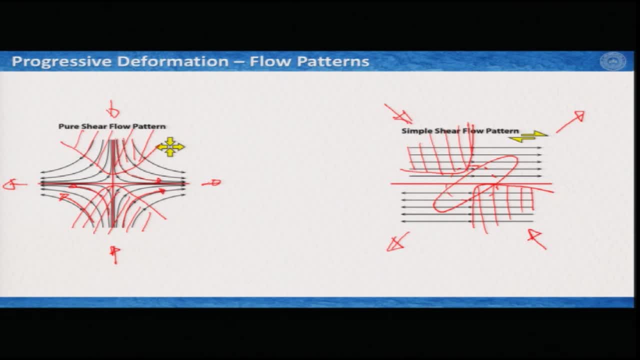 domain. Now, if you bring in between this combined pure and simple shear, then it would look like this: Here I have both symbols for pure shear and simple shear. What we see here that, unlike pure shear, here the material lines initially have some sort of compression, but then again they flow towards. 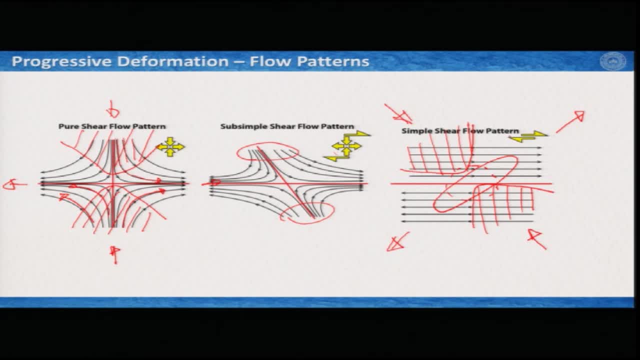 the extension and try to achieve something that we see in the simple shear pattern. Now, here again, it probably would have a compression. We would have a compression direction in this side, as you can see here, or compressive domain like this, and these are extensive domain. 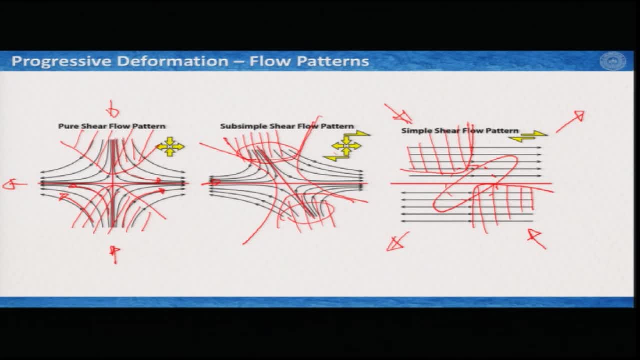 Now, because I have compression from one side and extension on the other side and also all materials. as you see that in these three very basic examples, they tend to flow towards the extension direction. From here, If I consider a material is sitting in between or a, then it may have a rotation or it may. 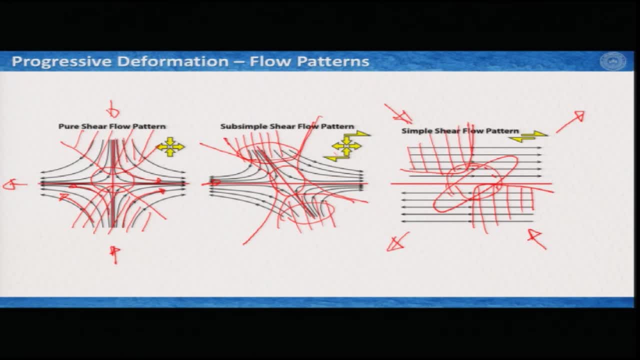 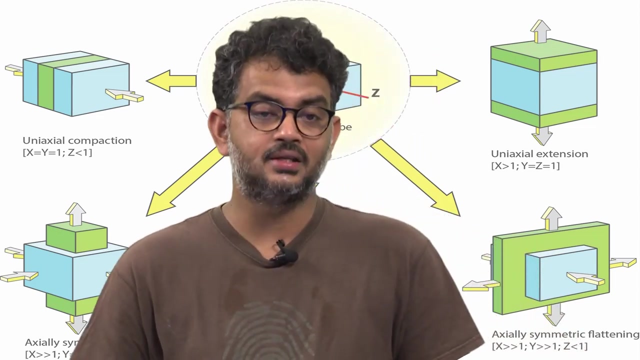 stay stationary. So, based on the flow pattern and nature of deformation, if we try to analyze whether the materials would stay stationary or materials would rotate, based on this study, we can go to another topic, which is known as vorticity. So vorticity is actually the study of, or it describes how, first a particle do rotate. 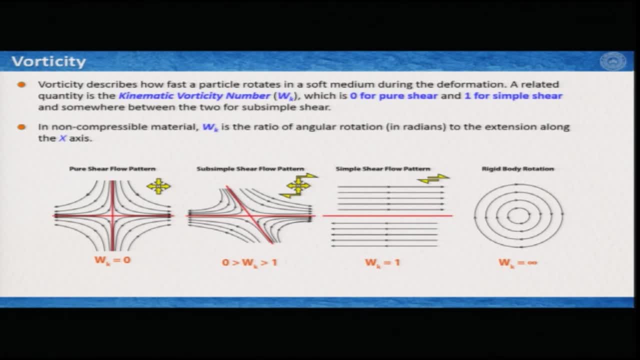 in a soft medium during deformation, and there is a term which is known as Kinematic vorticity Number. in mathematical expressions it is expressed as w? k and w k is as I said. it is Kinematic density number is assigned for pure shear as 0 and 1 for simple shear. So whatever. 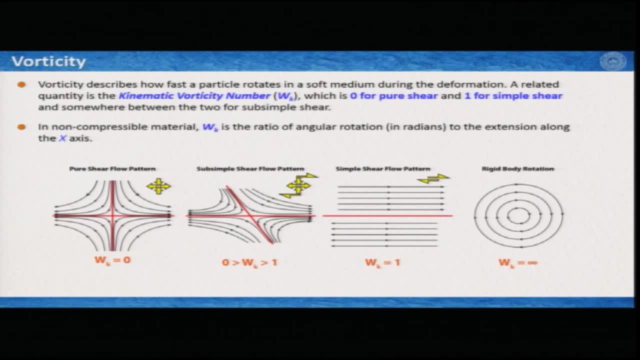 stays in between is a combination of pure shear and simple shear. So again we can have a look of the same diagram: that here Wk is 0. So this is pure shear. here Wk is 1, this is simple shear. and whatever stays in between from 0 to 1, this is your sub simple shear. 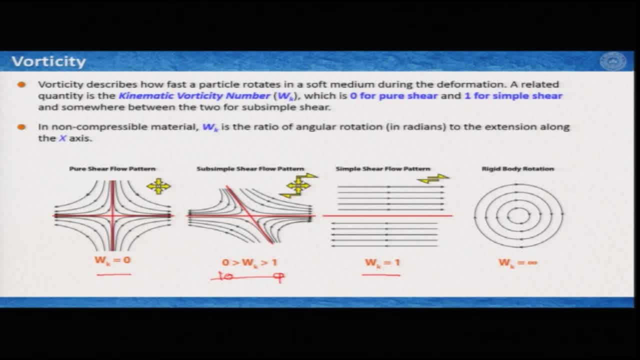 flow pattern, And if I increase the Wk value, then actually I achieve something which is whose flow pattern is very similar to rigid body rotation, and we see the effects of rigid body rotations in many different geological structures, So including the shear zone, features like delta structures. we have seen it one in one. 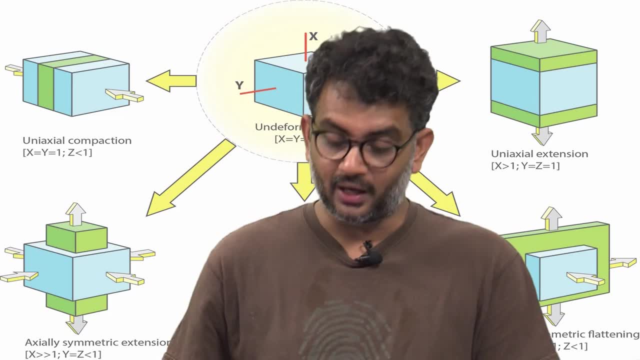 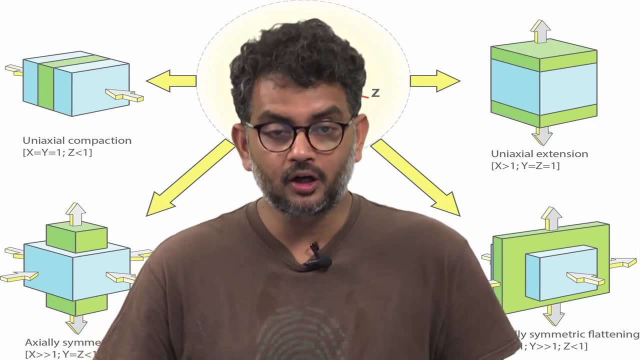 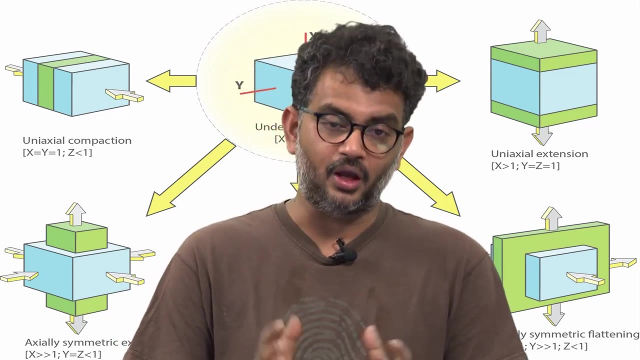 lectures, and we will see it more in when you, when you, study ductile shear zone. Now I conclude this lecture, but before concluding this, it is important to remind you that all these strain and deformation that we have learnt so far, these are just not the descriptions. 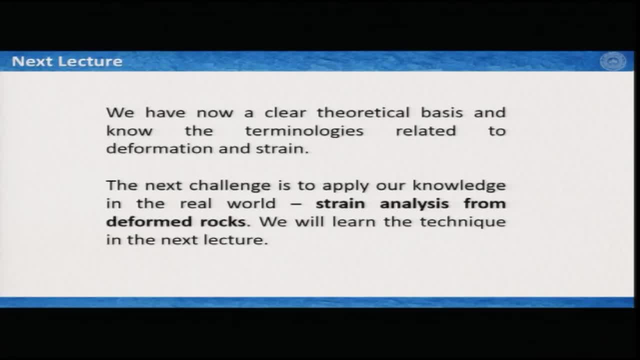 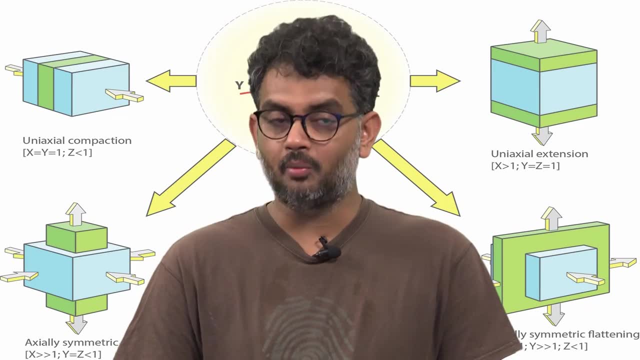 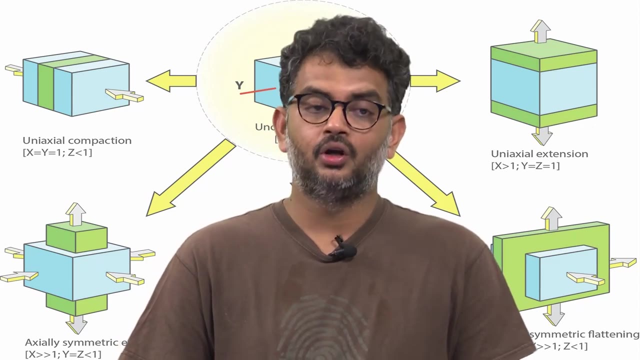 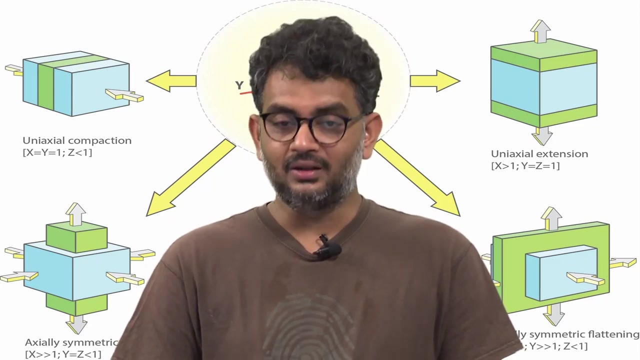 These include a mathematical analysis, which is not the scope of this lecture series, but I recommend you to read these books I recommended and also look and search in the web to have at least some basic ideas of the mathematical descriptions of strain. So in this lecture I believe, and together with the previous lecture, we have seen that 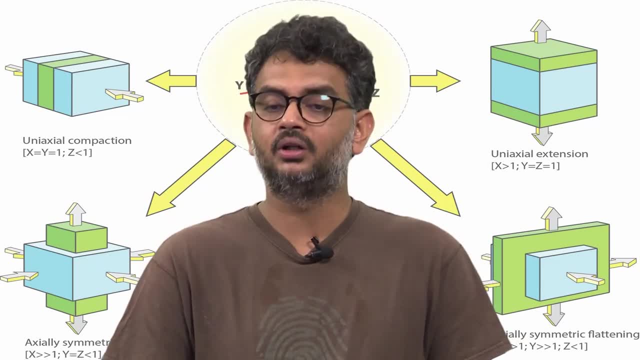 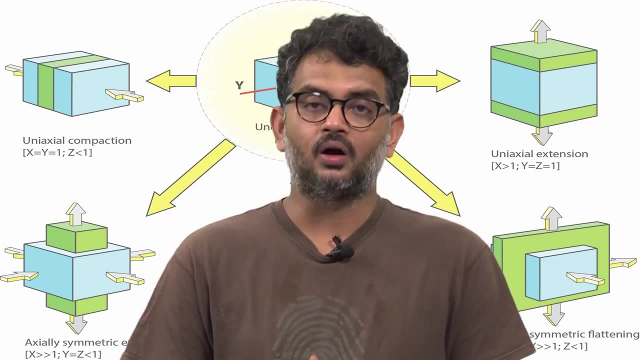 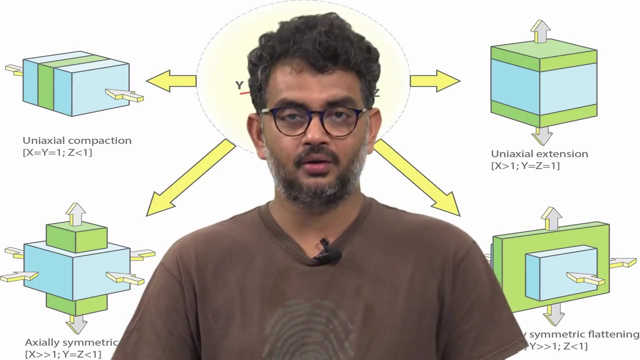 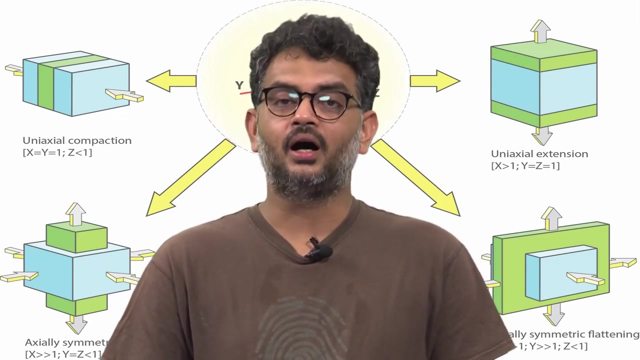 have some sort of theoretical basis and more or less know the terminologies that we deal with deformation and strain, particularly in the context of structural geology. Now the challenge is how to apply this knowledge to the natural field. That means if I see a deformed structure, then how to analyze or how to get strain or how to measure strain.